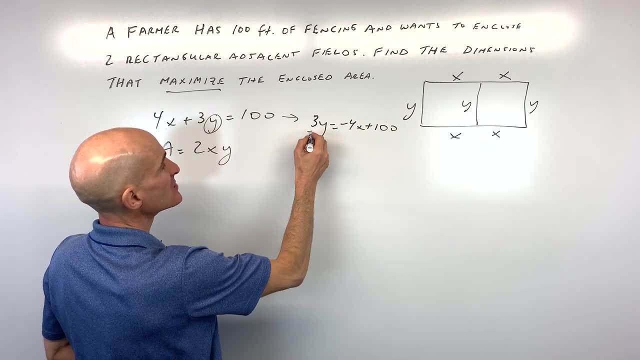 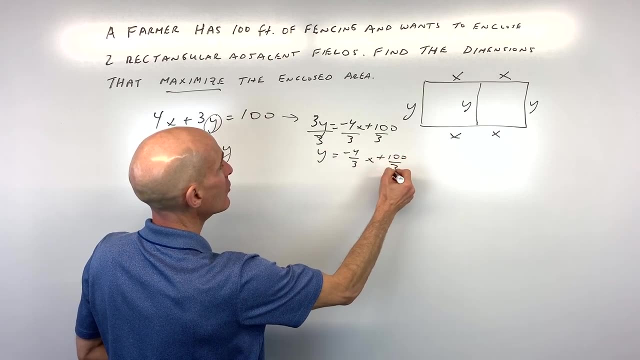 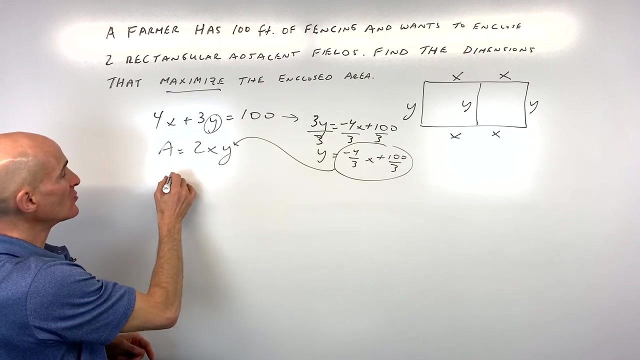 equals negative 4x plus 100, and let's divide everything by three, so that gives us: y equals negative four thirds x plus 100 divided by three. so now we know what y equals. we can then substitute or put that in place of y here, so let's go ahead and do that, so area equals. 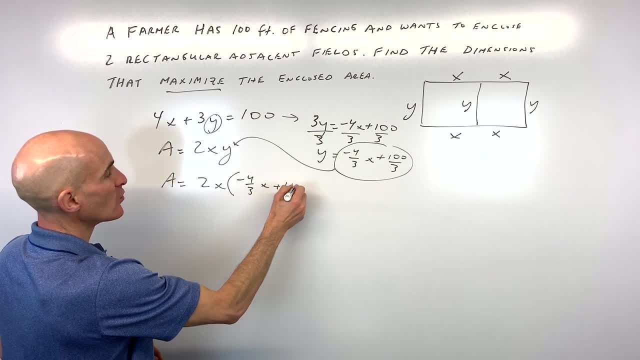 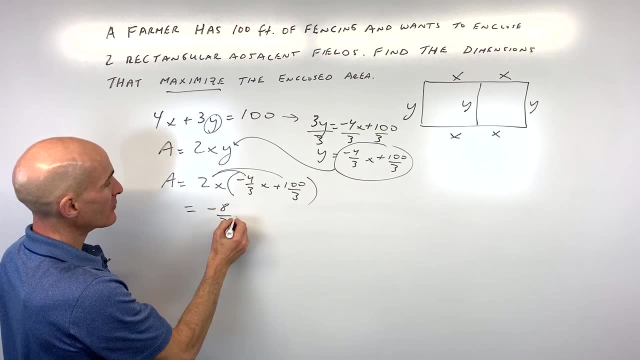 2x. negative four thirds x plus 100 over 3. and now what we're going to do is we're going to distribute the 2x and let's see what that gives us. so it's negative eight thirds x squared, plus 200 over 3 x. 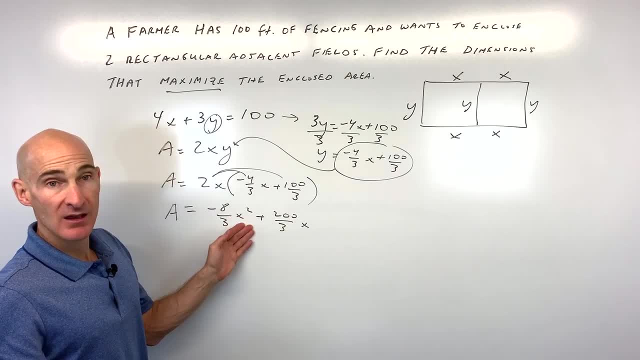 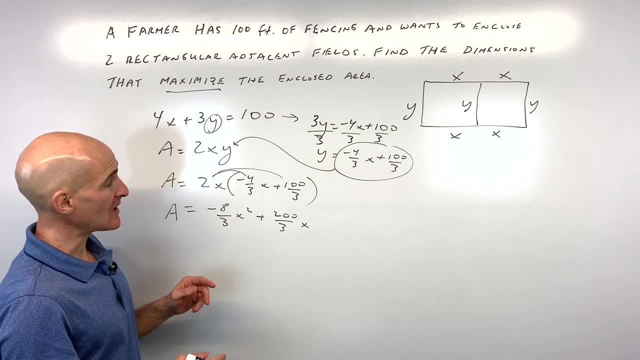 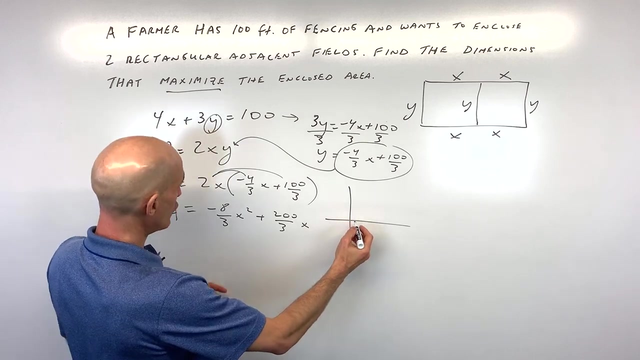 now what you can see is we have the area in terms of x and you notice that that's a value. this is negative. that tells us: this is a parabola that's opening downward. so if we were to graph this- and you can do this on your, on your graphing calculator by hand if you want- it's going to look. 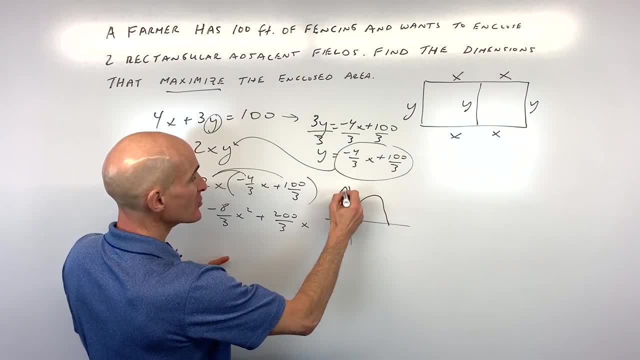 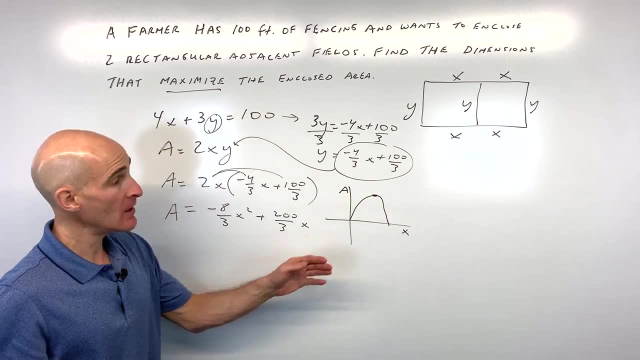 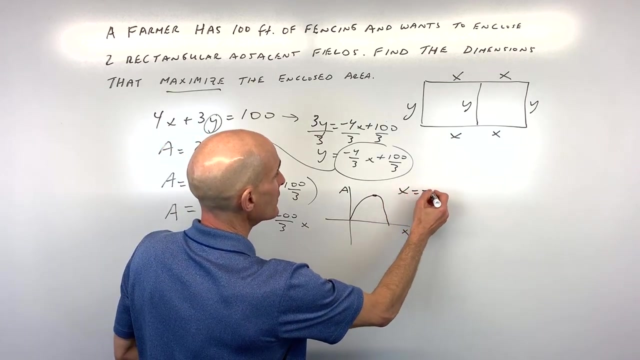 something like this: so here's your area, and in terms of x. so you can see we're looking for this point here that's going to maximize the area. notice that's the vertex of this quadratic, the vertex of this parabola, and remember to find the vertex we use this formula: negative b over 2a. so 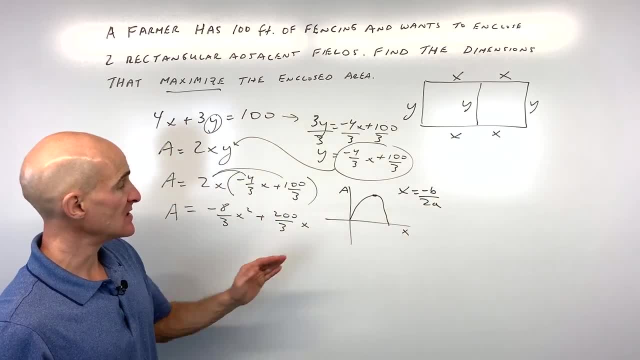 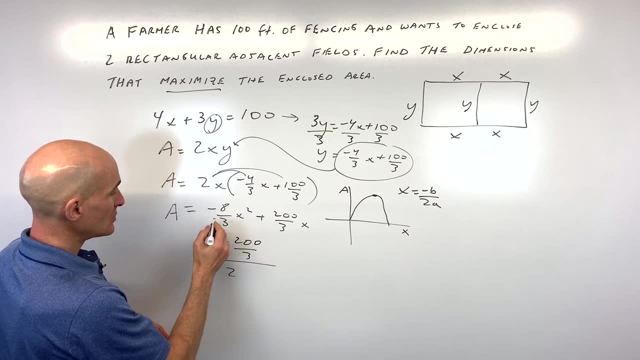 we're going to use this formula to simplify this, and then we're going to do this on the other side. So we've got A, B, C is 0. So the opposite of B would be negative 200 over 3 divided by 2 times A. 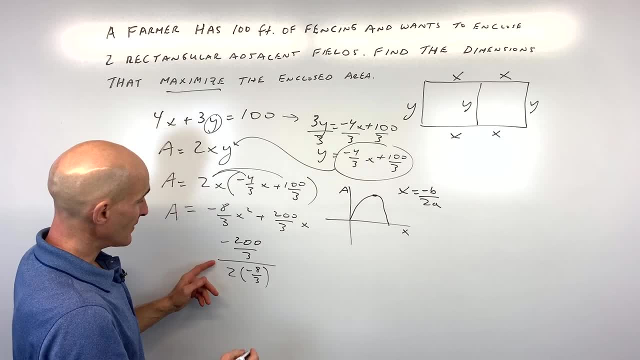 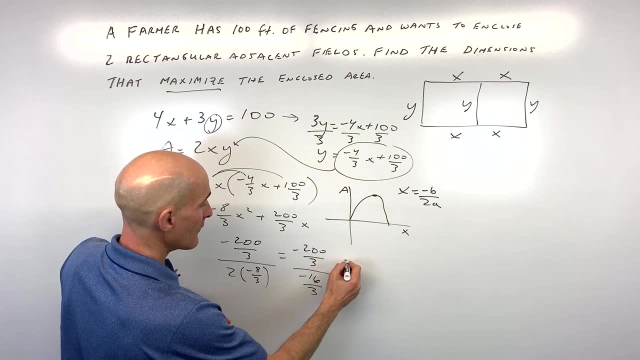 So 2 times negative, 8 thirds. Now simplify a little bit further. So this is negative 200 over 3.. This is negative 16 over 3.. If I multiply the numerator and the denominator by 3, that gives us negative 200 over negative 16.. 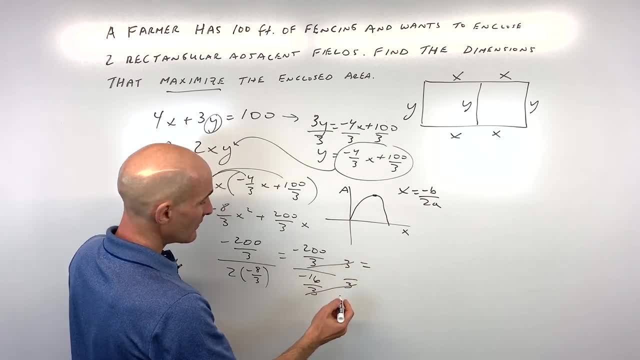 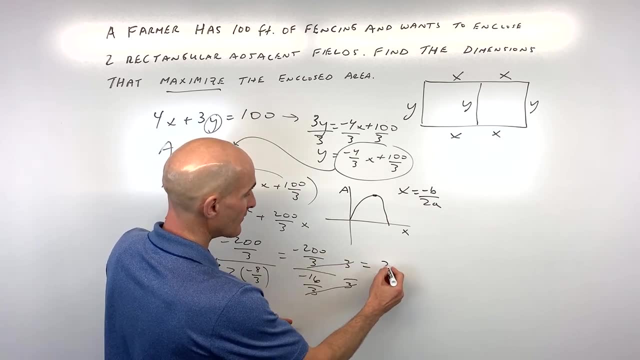 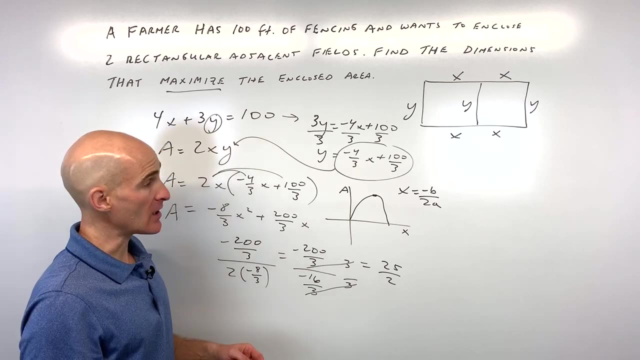 The two negatives cancel And if we reduce that down, that comes out to: let's see: 8 goes in here twice and 8 goes in here 25 times, So it's 25 over 2.. So that means when x is 12 and a half, that's going to maximize our area. 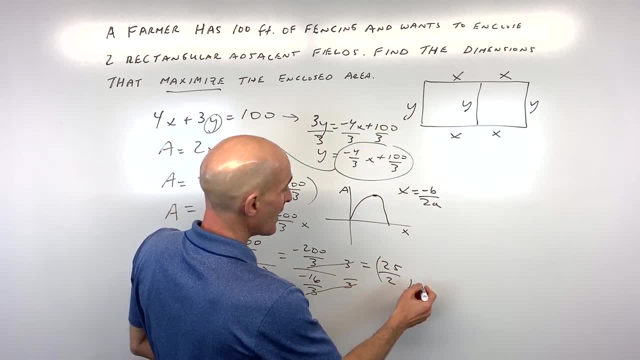 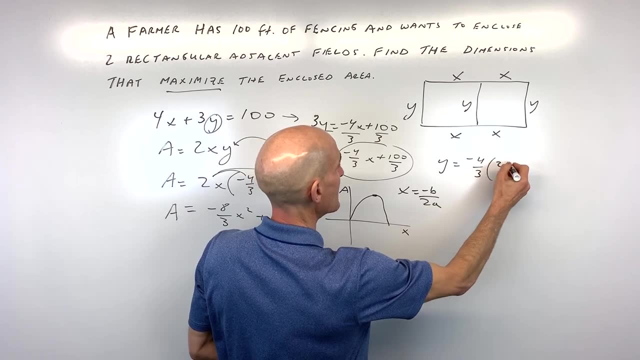 But let's find out what the other dimension is, y- And I'm going to do that by putting this back in for x here. So we have: y equals negative 4 thirds times 25 over 2 plus 1.. So that's going to give us negative 100 over 3..